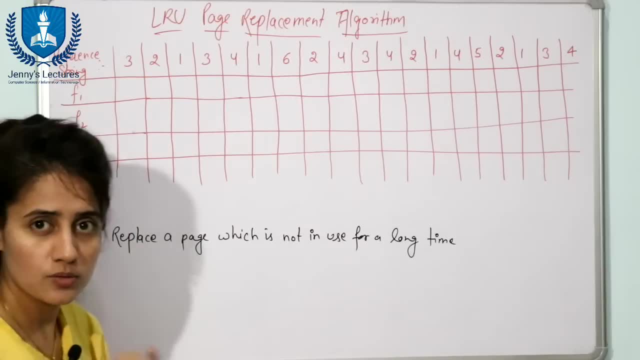 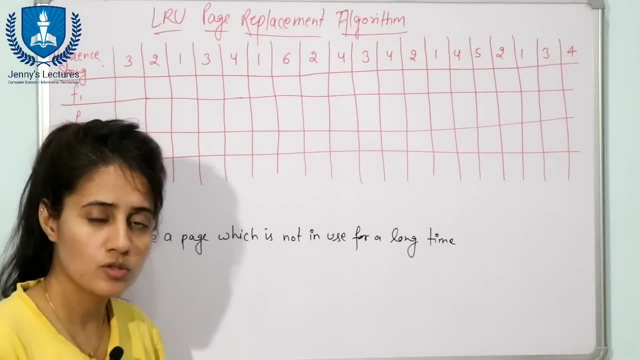 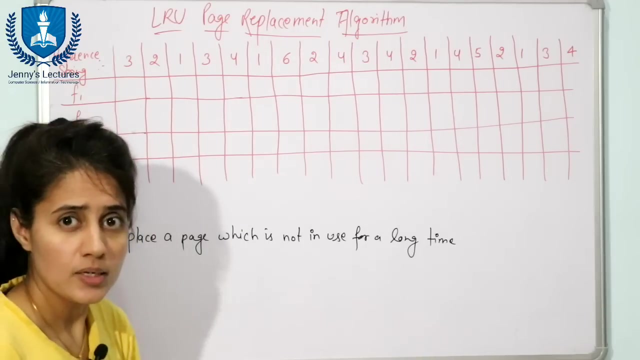 And we are given 3 frames: 1,, 2 and 3.. Now you have to apply LRU page replacement techniques and you have to find out the number of page faults plus you can say that hit ratio Plus in question. they can also give you one more condition, that when all the frames are empty. 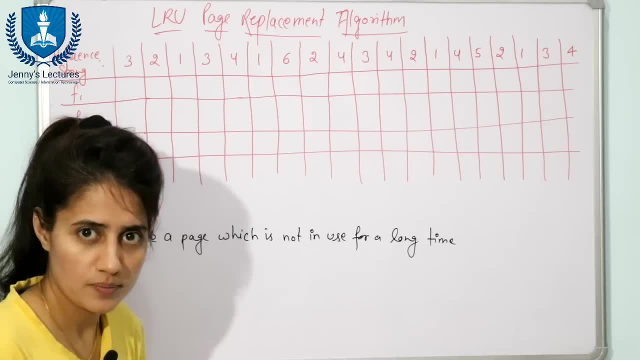 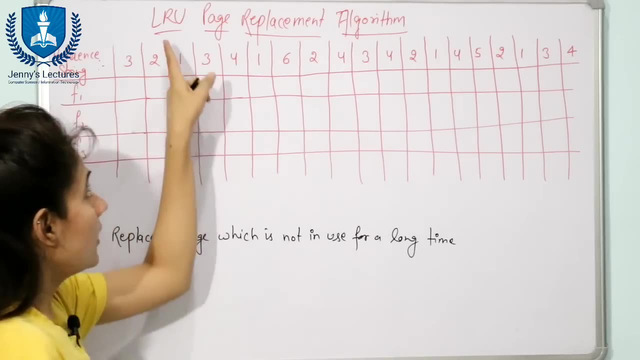 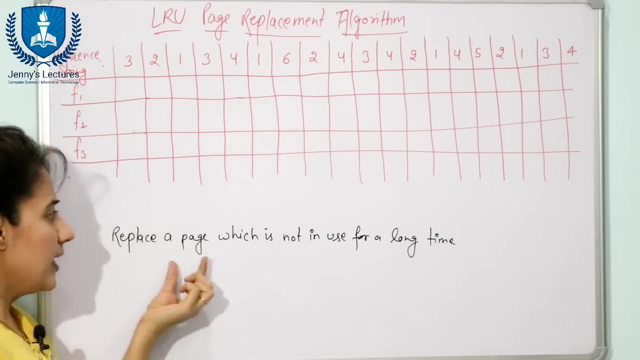 then also it would be considered as a page fault. Okay Means in starting, because all the frames are empty, we have no page. Okay, See Now what is this? LRU? page replacement techniques. It means least recently used. Or you can say replace a page which is not. 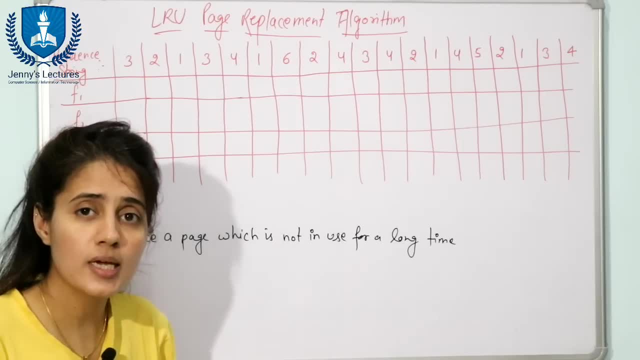 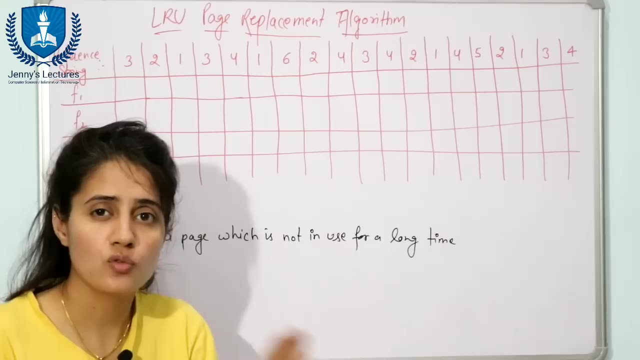 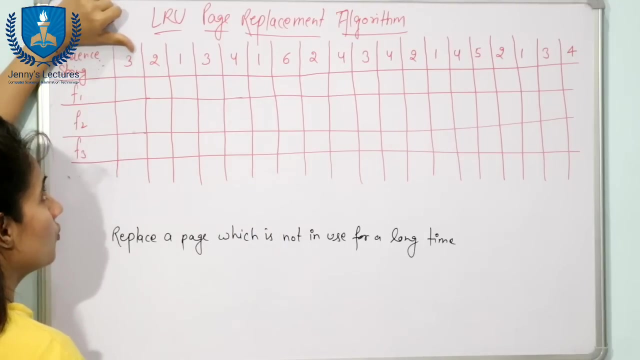 in use for a long time. Or in other words, you can say: we are going to replace a page that has not been used for the longest amount of time. Okay, Now how to apply this technique: See The first CPU has requested for page number 3.. We have 3 frames We don't have. 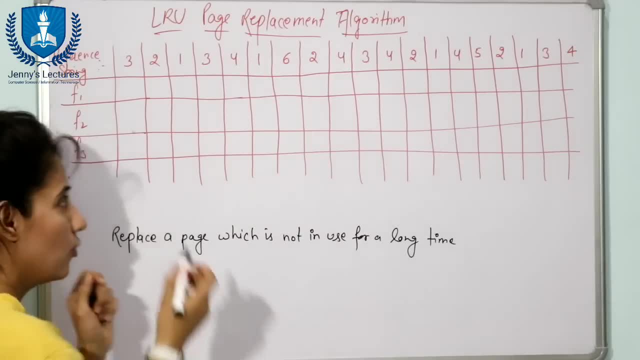 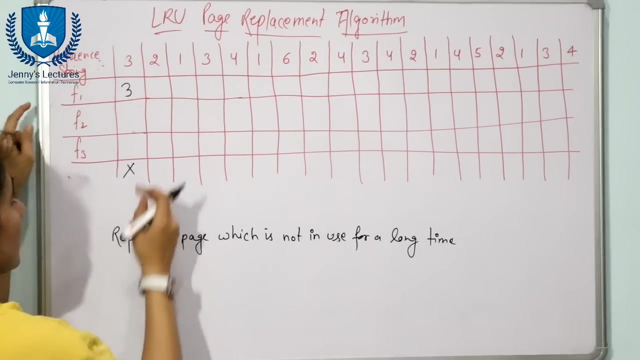 the page number 3.. So this means it means it is a page fault, Means we are not having this page. Now we will store this page in frame 1.. You can start inserting these pages from here also: F1,, F2,, F3. Like this: Okay, That is also fine. Next page is page number 2.. Check out. 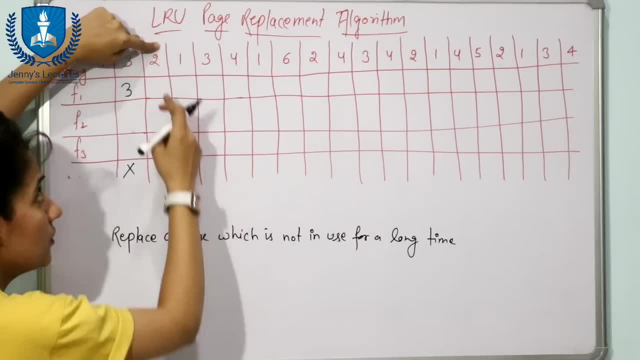 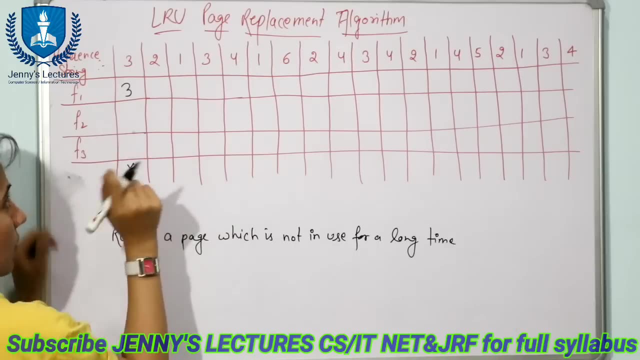 Do we have this page number? Operating system will check if this page number is available in the main memory, Because main memory is divided into frames- See No. 2 is not available, Only 3 is available. So we will store this 2.. We will load this 2. And this is also a. 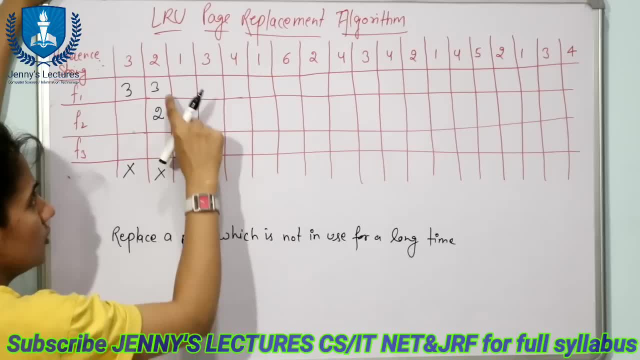 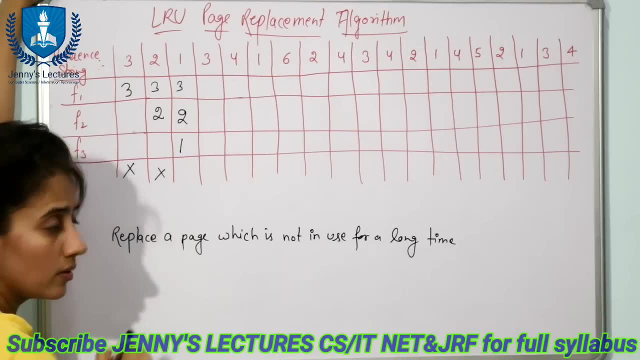 page fault Means this page is not available. Next is 1. Check No. 1 is not available, But 1 frame is free, So we will put 1 here only. Okay, And 1 was not available, So this: 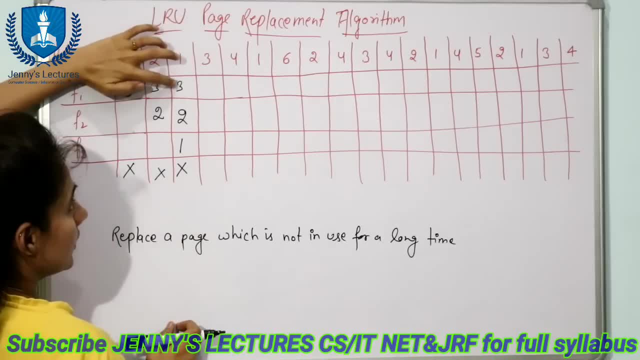 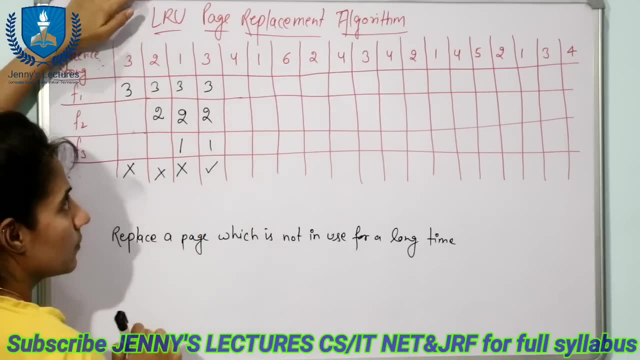 is also a page fault. Now request is 3. Now check: Yes, This page is available in our 3 frames, So this is a hit. 3,, 2, 1.. Next is 4. Check out: 4 is available. No 4 is. 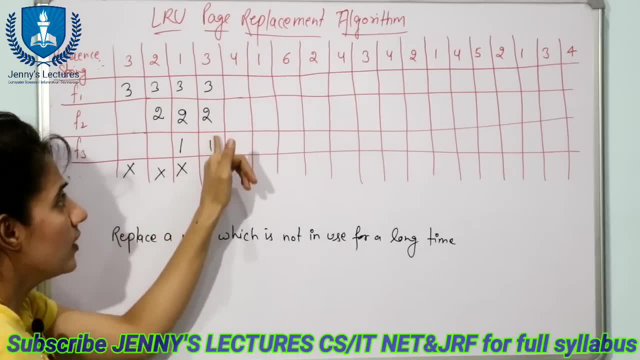 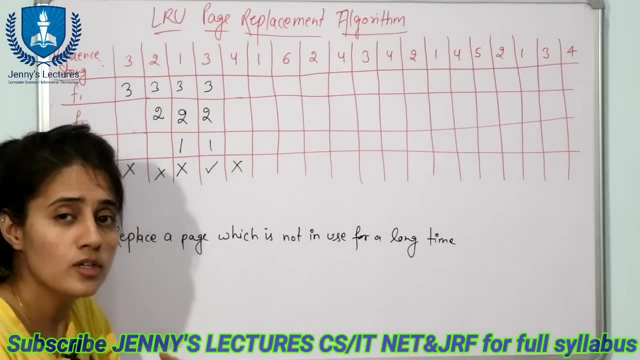 not available, So this is a miss. Now all the frames are full. We cannot put this 4 here. now what you have to do, the operating system will choose one page from here and this page is to be swapped out in the secondary memory, and this page, number four, is swapped in in this main memory. 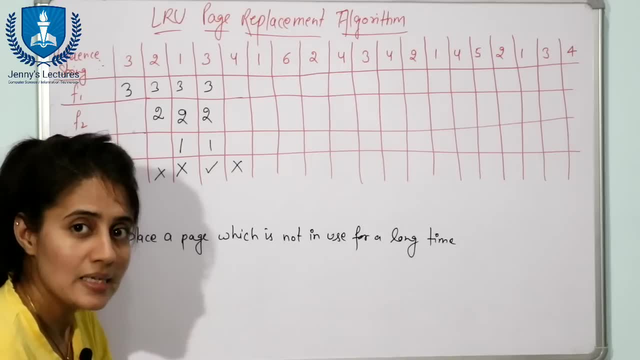 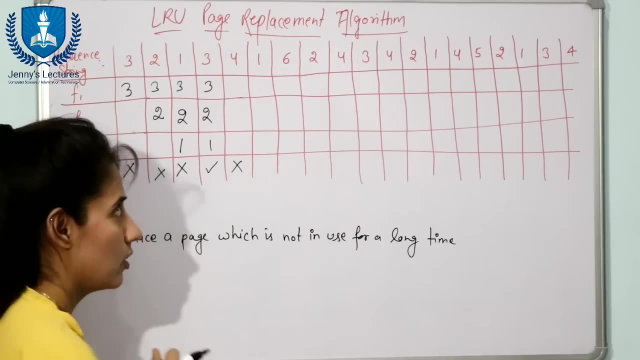 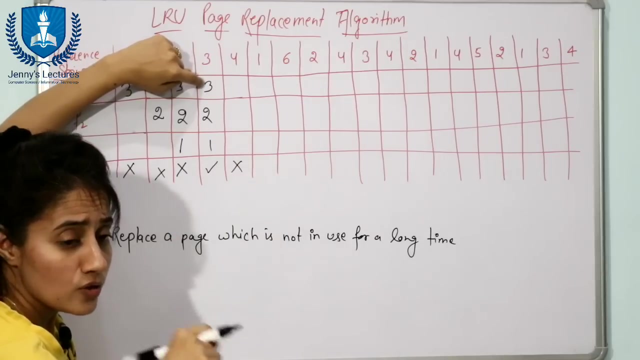 now which page is to be swapped out. that is taken. that criteria is taken care by this page replacement technique that is lru least recently used. now check out out of these available pages which page is least recently used, or you can say which page has not been used for a long amount of. 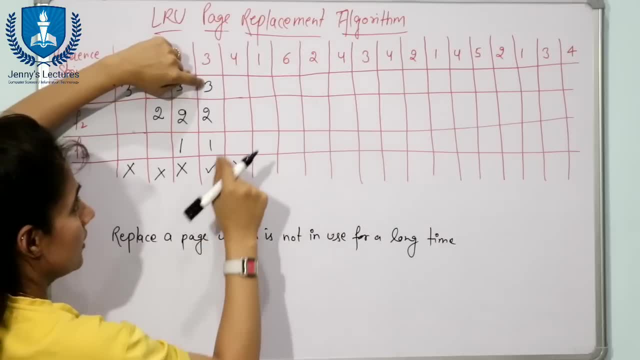 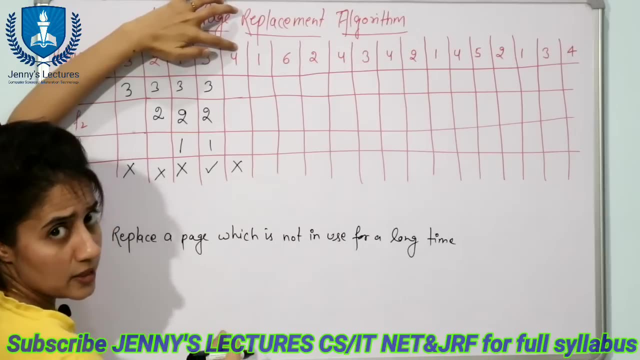 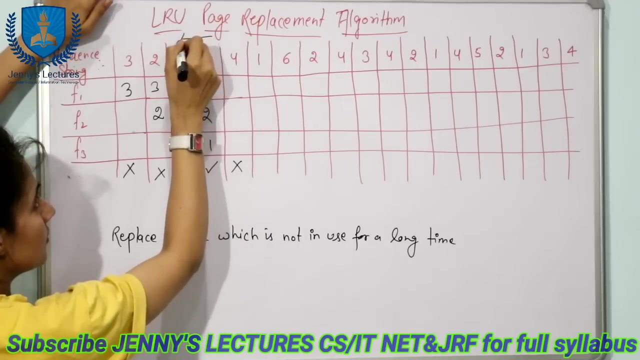 time for the longest amount of time. okay, how you will check, see, the simple trick is here. this is for I am going to swap in this page for now. from here we will trace out this reference string from right to left like this, fine, and check see. three, two, one, three is here means 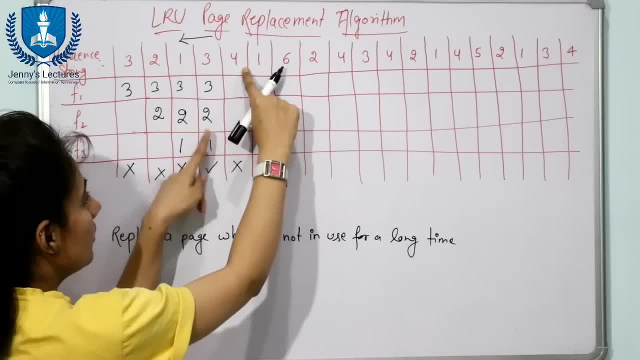 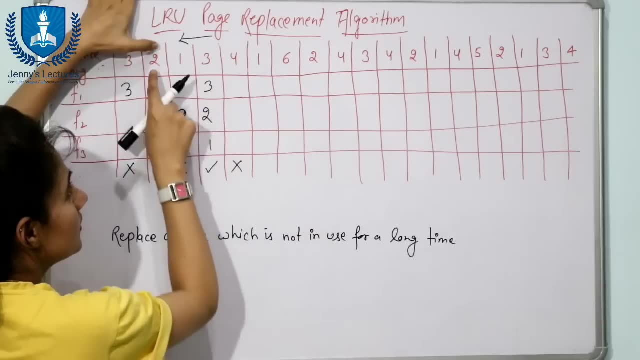 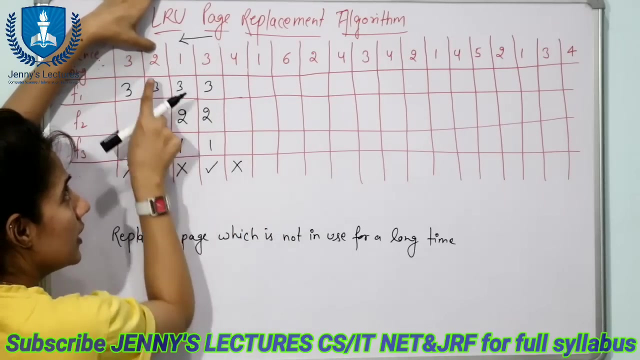 recently used is three, then one and then two. it means the least recently used page is two. why? because this two is to the left, more to the left, most side of all the three pages available in the frames. it means we will choose this two, we will replace this two and put four here. three: 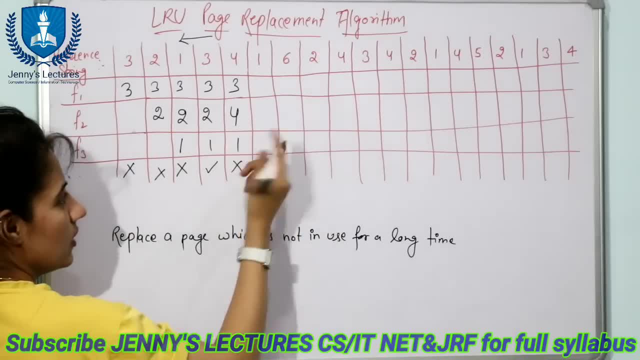 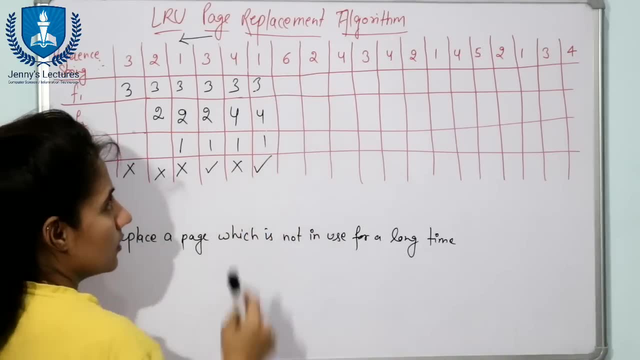 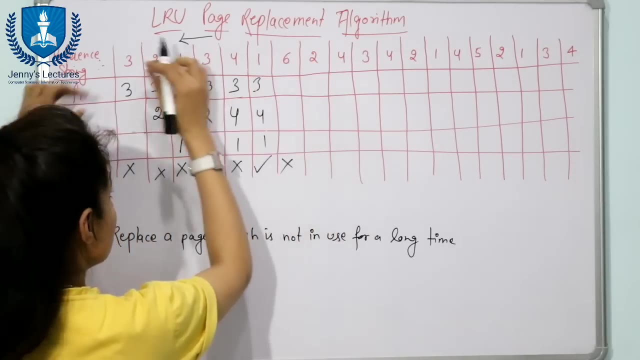 and one. let's check out for another one. one one is available, so this is a hit. three, four. now. next is six. three, four. one. six is not available, so this is a miss. now which page is to be replaced from here? we will trace out this string from right to left, okay. 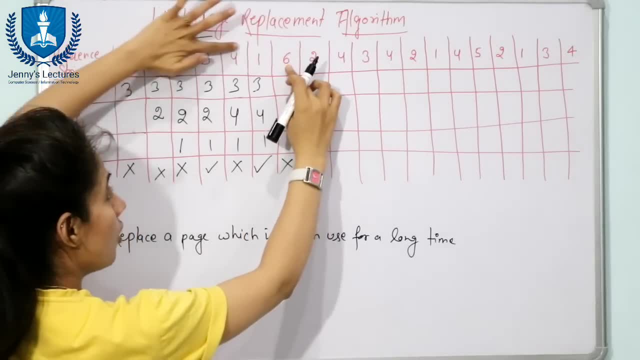 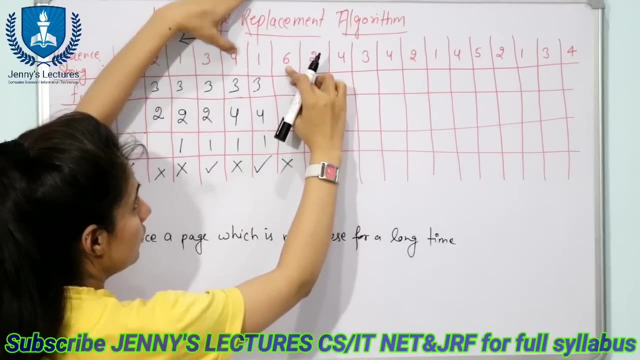 because we are going to see in the past which page is not being used for a longest amount of time out of available pages, three, four, one. see here we have one, here we have then four, then we have three. it means to the left most side out of these pages. which page is there three? 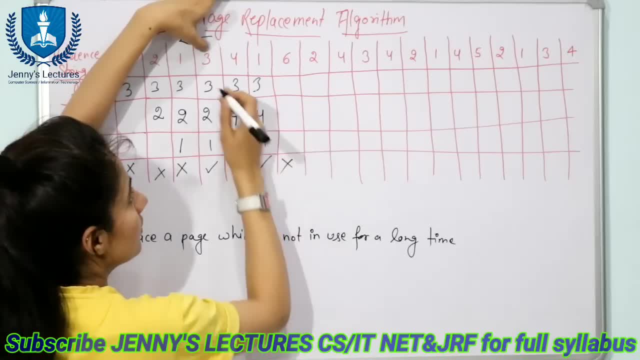 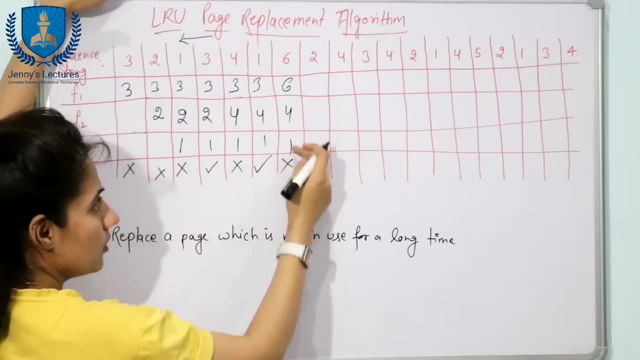 So we will choose this one. This is the least recently used. We will choose 3.. Here we will write 6,, 4 and 1.. Next is 2.. 2 is not available. It is a miss. Check out. 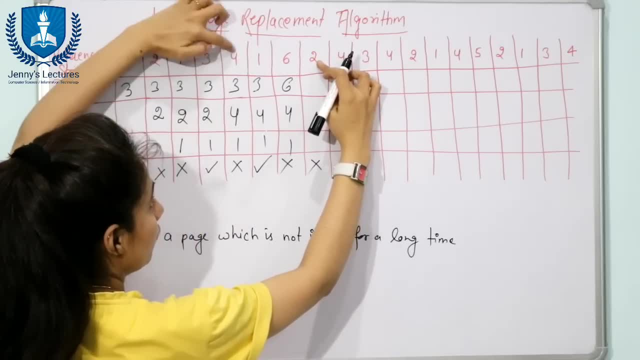 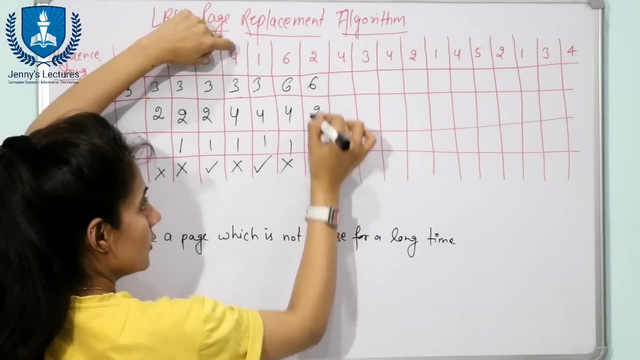 6 is recently used, Then 1., Then 4.. So to the left, most side of all the 3 pages, which one is Page is there, 4.. So we will replace this one, 6 and 1.. 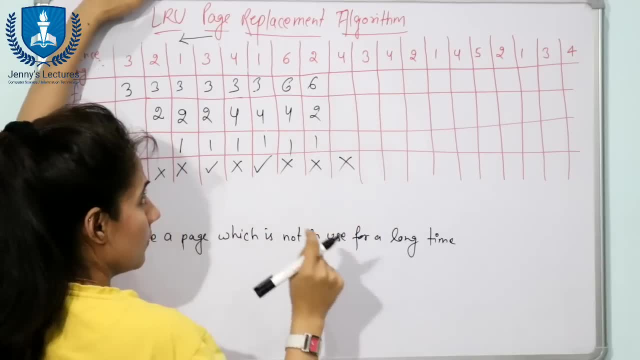 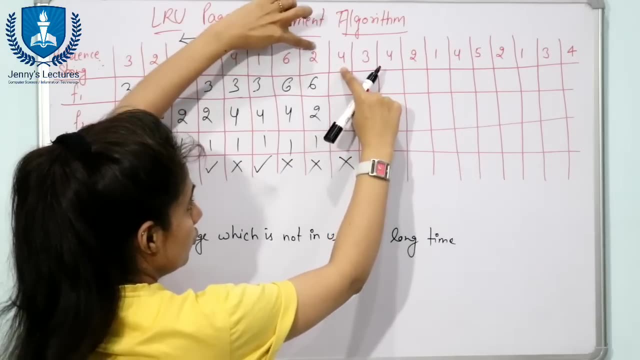 Next is 4.. This is a miss because 4 is not available. Now. see out of these: 3, 6,, 2 and 1, which is to the left, most side from here. 2 is here. Then we have 6.. 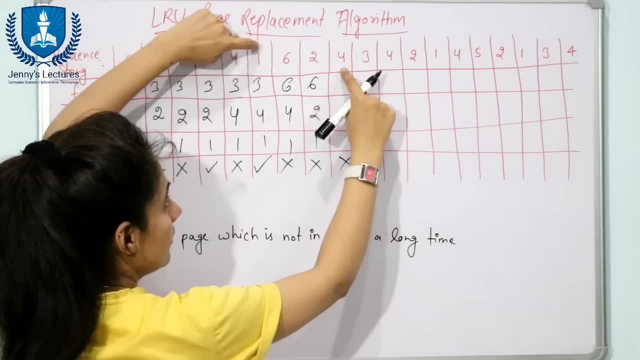 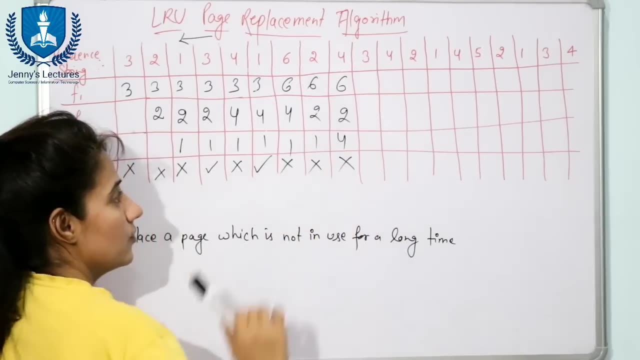 Then we have 1.. It means 1 is the least recently used. We will replace this: 1,, 2 and 6.. Next is 3.. 3 is also not available. Find out which page is to be replaced: 6,, 2, 4.. 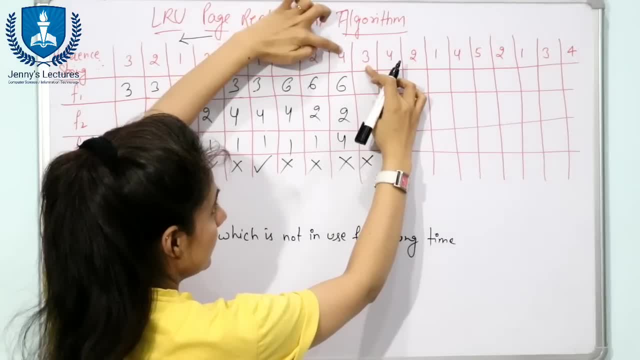 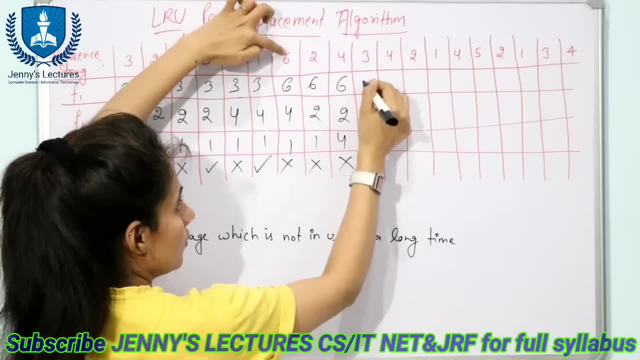 Out of these 3, which is the least recently used. 4 is recently used. Then we have 2.. Then we have 6.. To the left, most side 6 is there out of these 3.. So we will replace this 6.. 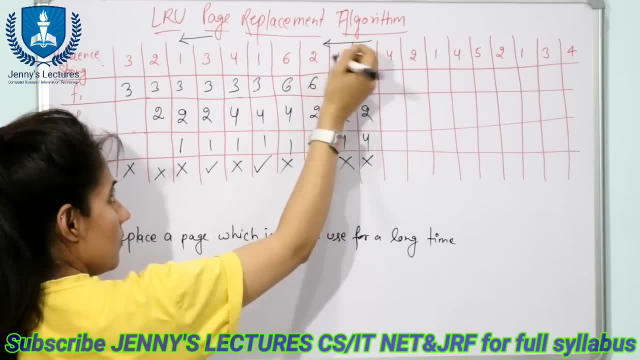 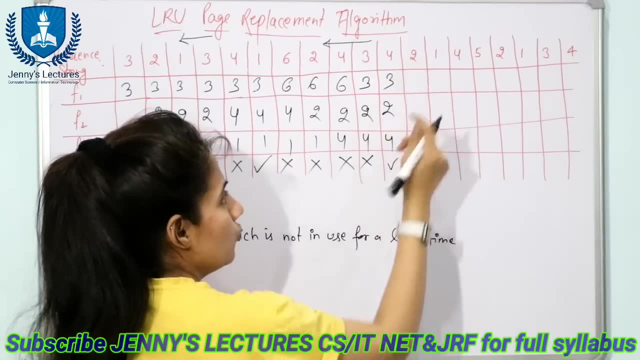 This is the simple trick. Just check out, Just trace out this string from right to left: 4. 4 is available. So this is a hit: 3, 2, 4.. 2. 2 is available. 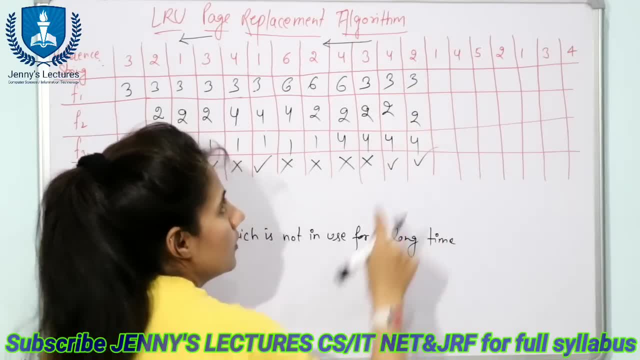 So this is a hit: 3,, 2, 4.. Now next is 1.. 1 is not available. 3,, 2, 4 are available. So this is a miss. This page is not available. 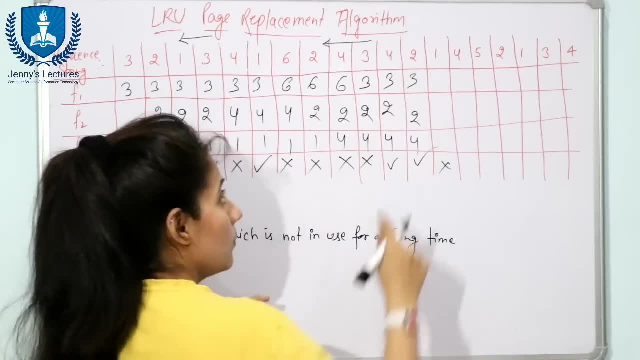 So next is: 1.. 1 is not available. 3,, 2, 4 are available. So this is a miss. 3,, 2, 4 are available. Now check out Which page is to be replaced. 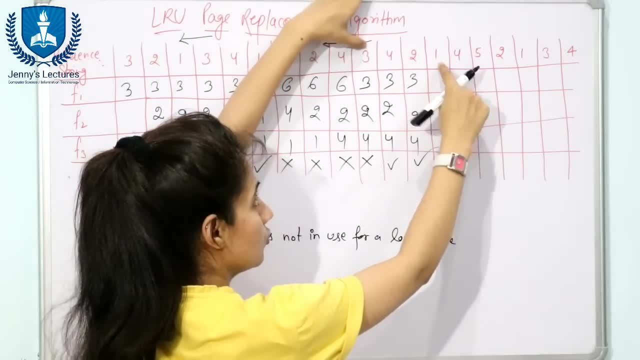 3, 2, 4.. Here we have 2.. Here we have 4.. Here we have 3.. So 3 is to the left most side 3 would be replaced 1,, 2 and 4.. 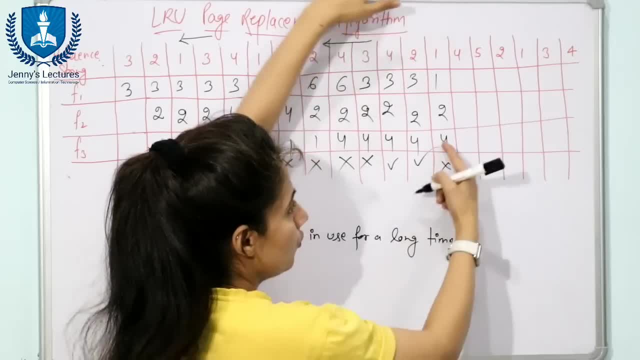 Next is 4.. 4 is available. So this is a hit. 1,, 2 and 4.. 5 is not available. This is a miss Which is to be replaced: See 1, 2, 4.. 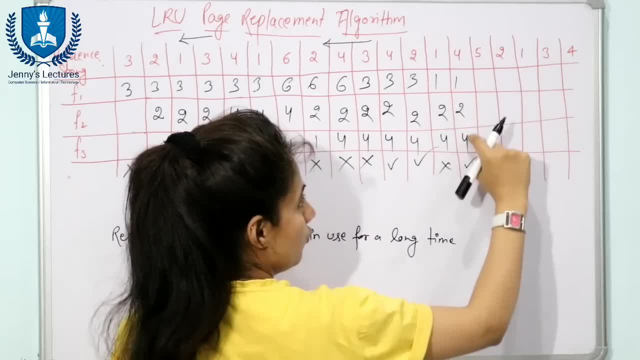 Out of these: 3. 4 is here, Then we have 1.. Then we have 2.. So we will replace this: 2. 5, 1 and 4.. Now check out Which page is to be replaced. 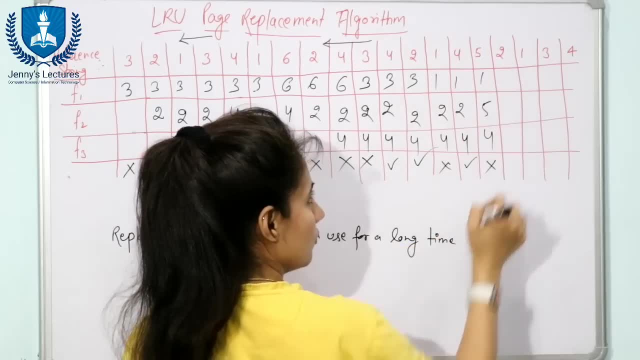 3, 2, 4.. Here we have 2.. 5, 1 and 4.. Next is 2.. 2 is not available, Which is to be replaced? 5 is here. 4 is here. 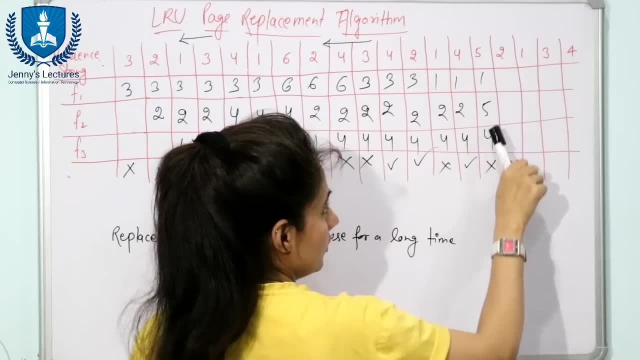 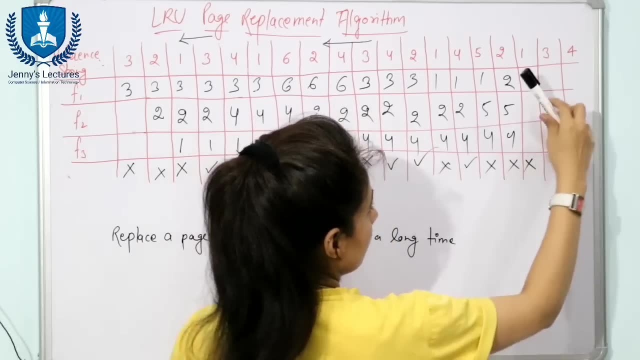 1 is to the left, most side of all these 3. So 1 is to be replaced 5 and 4.. 1. 1 is not available Now, out of 2,, 5,, 4.. 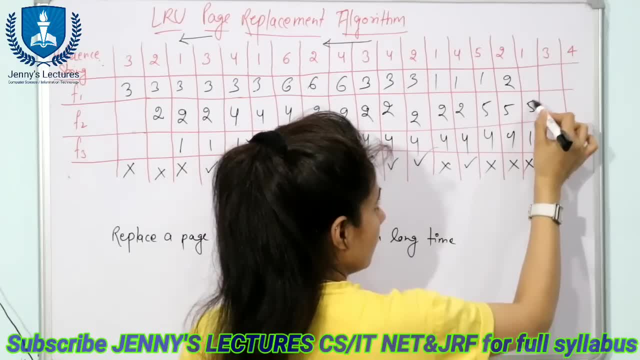 2 is here, Then 5., Then 4.. Then we will replace this: 4., 5 and 2.. 3 is not available, Then 2, 5, 1.. 1 is here. 2 is here. 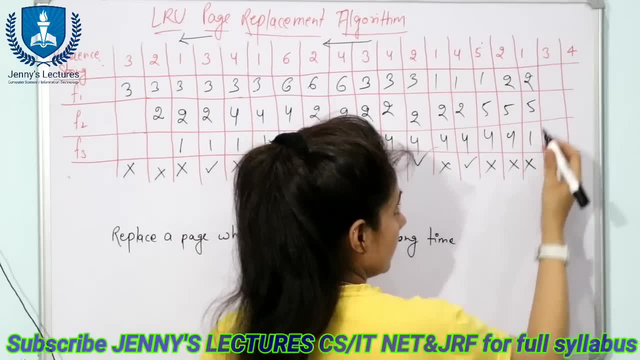 5 is here Left most side, That is, 5. Means: this is the least recently used, So we will replace this: 1. 2 and 1. 4 is not available, So you will replace what: 2, 3, 1.. 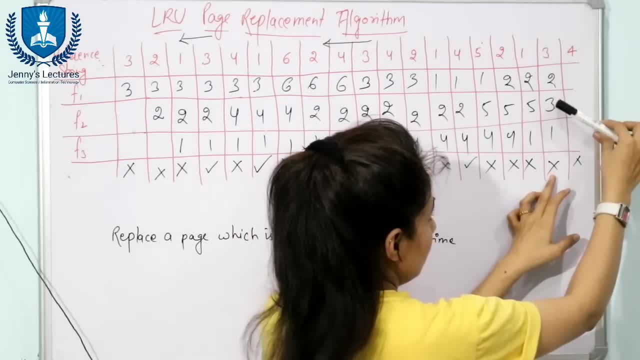 Out of these, 2,, 3, 1.. 3 is here, Then 1 is here, Then 2 is here, Then we will replace this: 2.. 4, 3 and 1.. So number of page folds are: 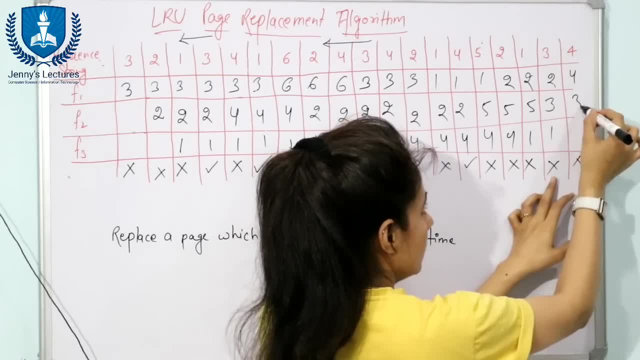 Check out: 1,, 2,, 3,, 4,, 5,, 6,, 7,, 8,, 9,, 10,, 11,, 12,, 13,, 14,, 15,, 16,, 17,, 18,, 19,, 20,, 21,, 22,, 23,, 24,. 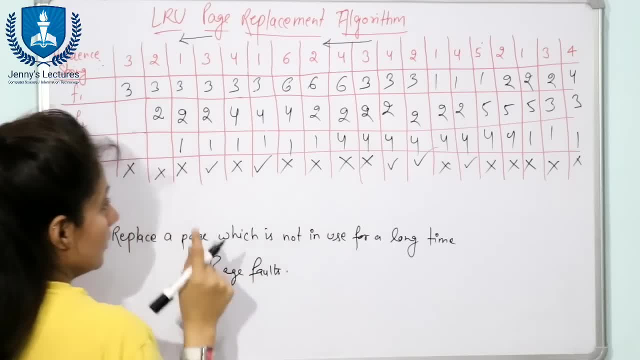 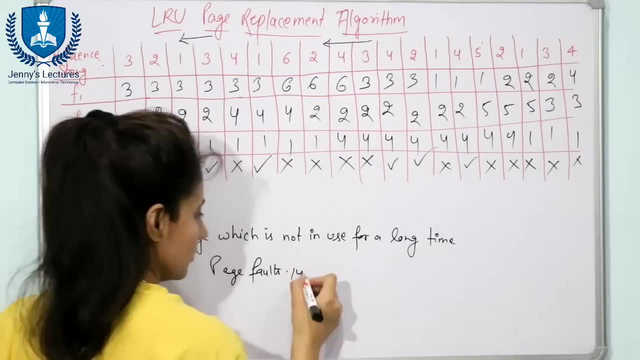 25,, 26,, 27,, 28,, 29,, 30,, 31,, 32,, 33,, 34,, 35,, 36,, 37,, 38,, 39,, 40.. If you are asked to find out the hit ratio, then how you will find out. 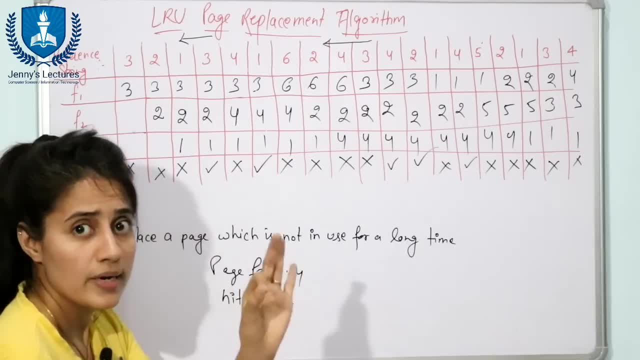 Check out number of hits: 1, 2,, 3, 4, 5.. 5 hits are there. Divided by total, Total is what? 90.. OK, So total is 90.. So total is 90.. 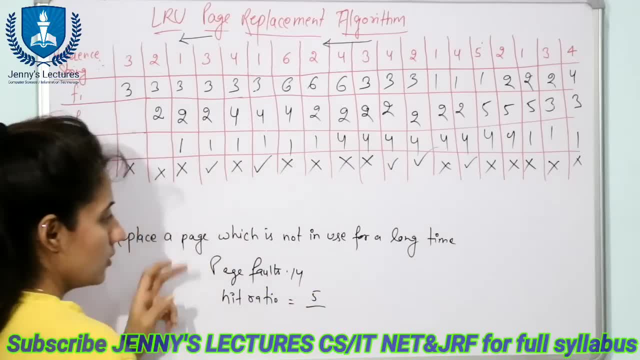 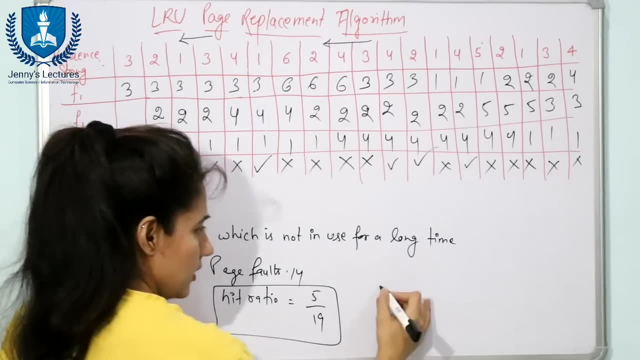 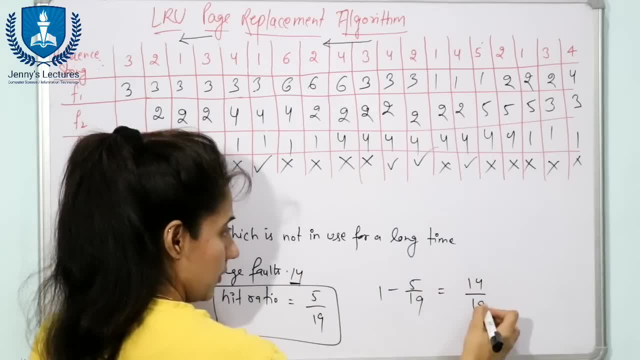 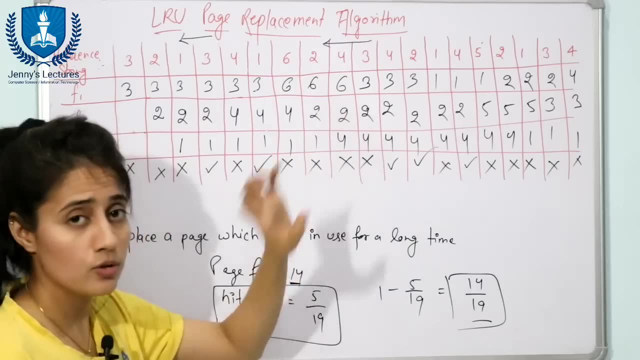 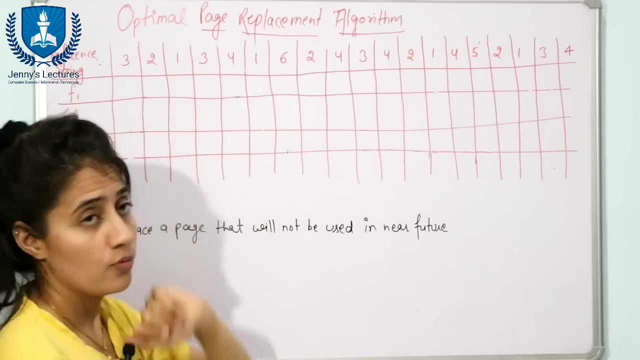 number of folds are these: So 14 divided by 19.. So this is the LIU technique. Now we will discuss how to solve this numerical only using Optimal phase replacement technique. So next is optimal phase replacement technique. We will solve this same Numerical with the help of Optimal phase replacement technique. 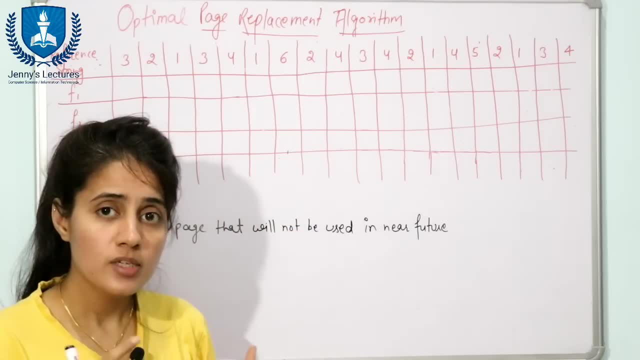 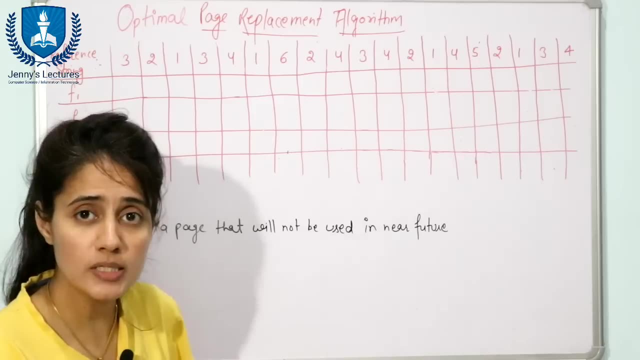 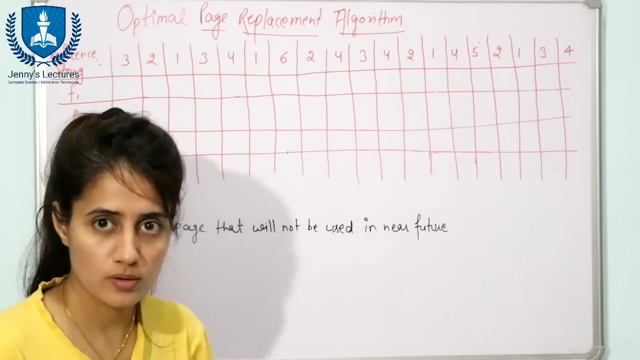 Now, what is this technique? What is the criteria area? see, in this case we will replace a page that will not be used in near future, or you can say that will not be used for the longest amount of time in future. so in this technique, we are going. 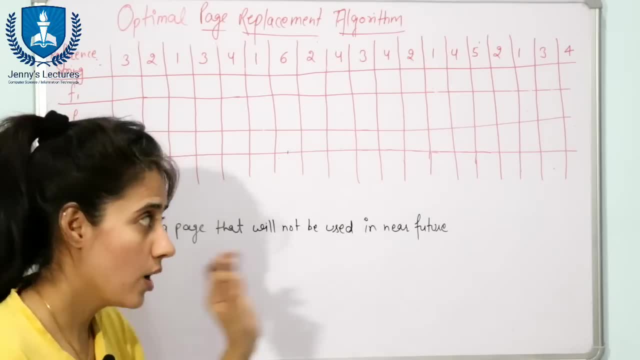 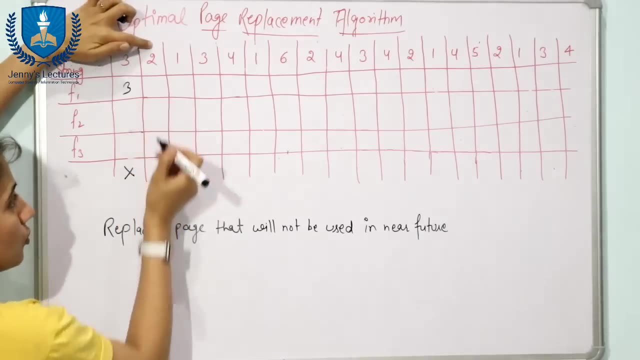 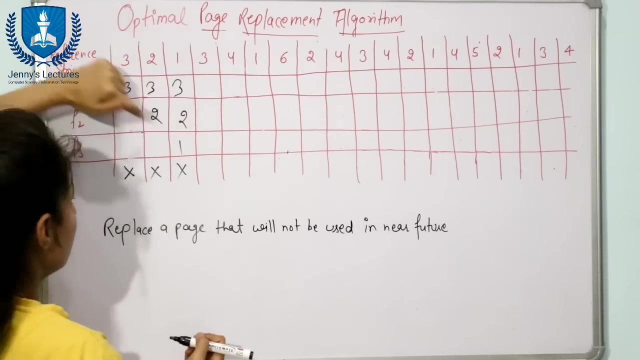 to take into consideration the future activity. okay, now how this technique is to be applied: see same. three is not available. this is a mess. two is not available, so this is a mess. we will load this. two: one is not available. this is a miss. three, two and one. all the frames are now full. 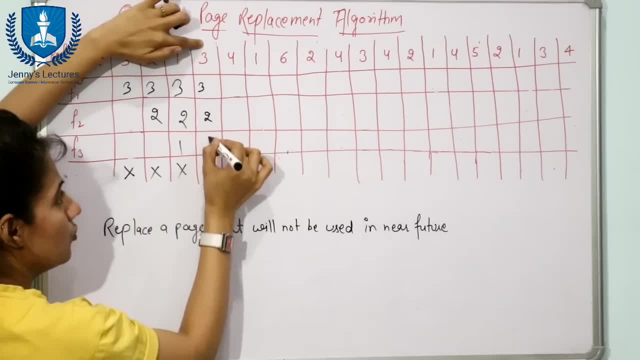 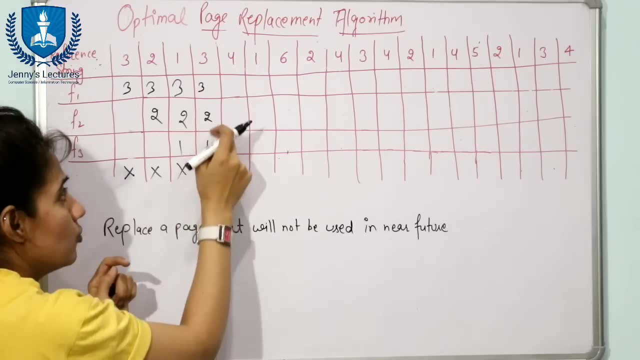 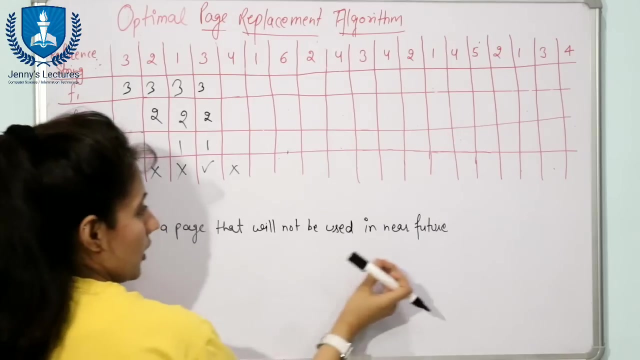 now three. three is available, so this is a hit: three, two and one. now four, see, four is not available. so this is a mess. now, which page is to be replaced? which page is to be selected as a victim page? which page is to be swapped out into secondary memory? check out, see, we are going to take into. 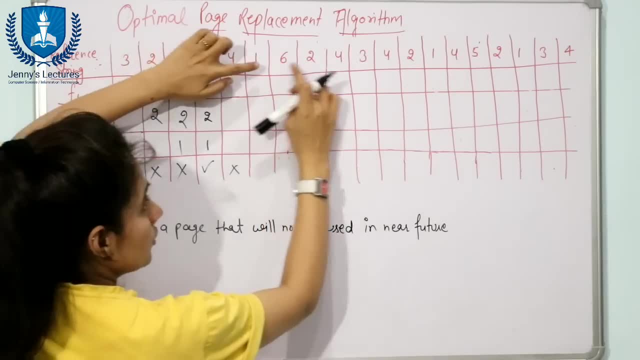 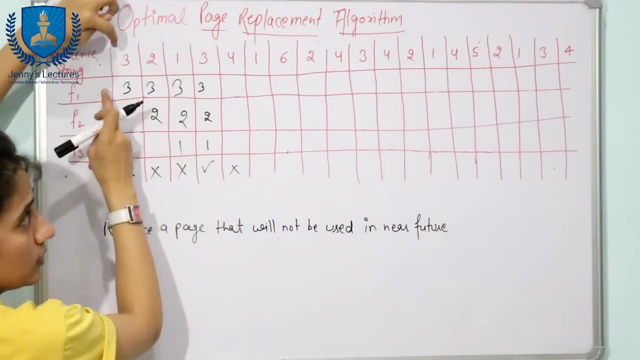 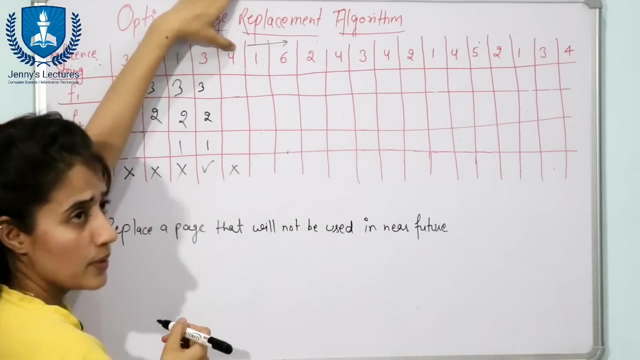 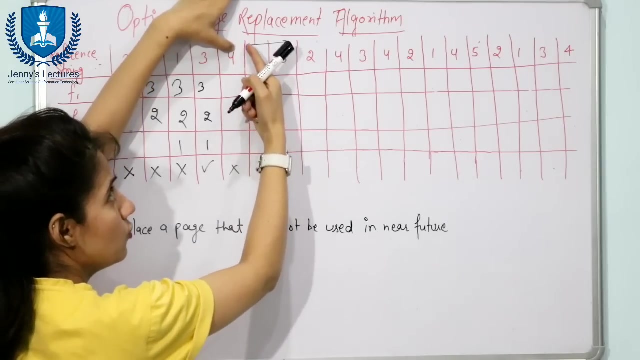 consideration, consideration the future activity. so future is the side in lru we have. we have taken into consideration consideration the past activities. so now we will re, we will trace out this reference string from left to right. we are going to put this page now. cpu has requested this page. so from this page from you can say, from this page we are going to trace. 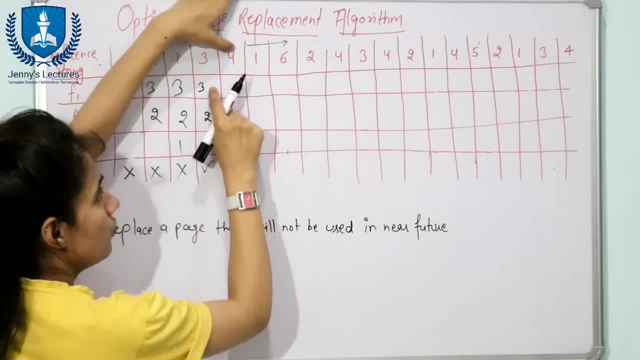 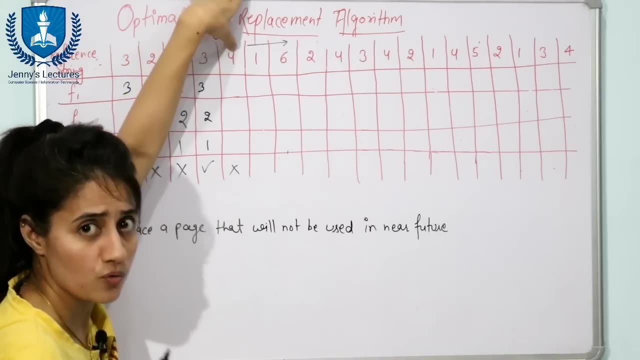 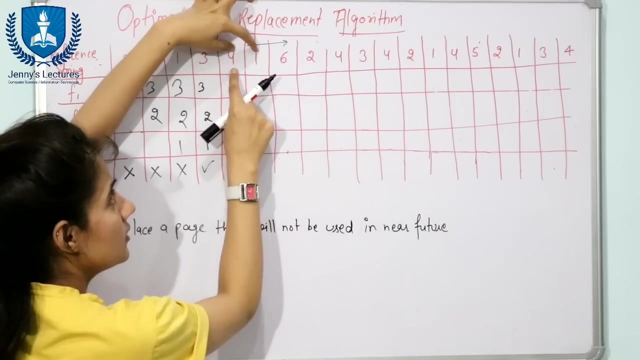 out the string from left to right. now see out of these pages, available pages. which page is not going to use for the longest amount of time in future? check out one. one is available here so we can say that after this request, cpu will request for this one, so we cannot replace this one. 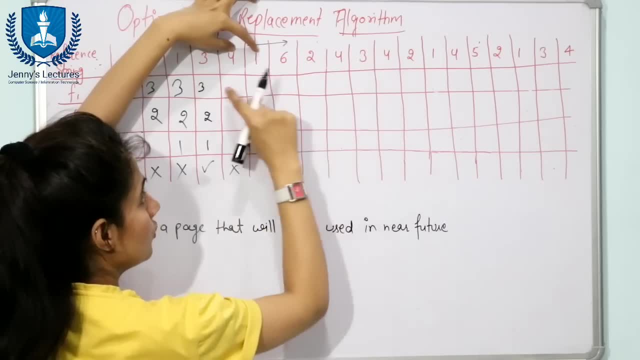 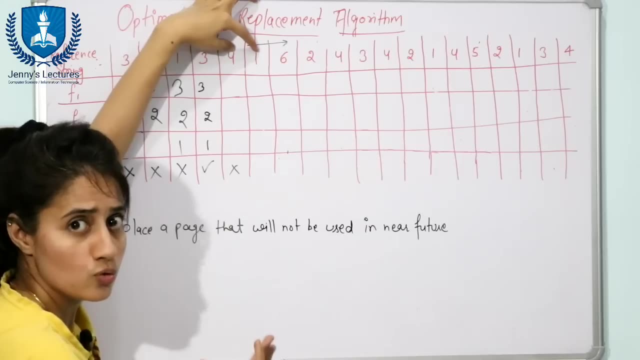 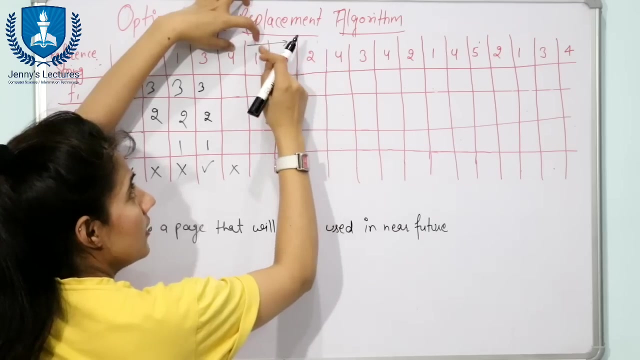 then cpu will request request for two, then cpu will request for three. so this is: this page is to be selected as a victim page. this page is not going to be used in the future, in the near future, you can say okay. so the simple trick is just trace out from left to right and the page which is to 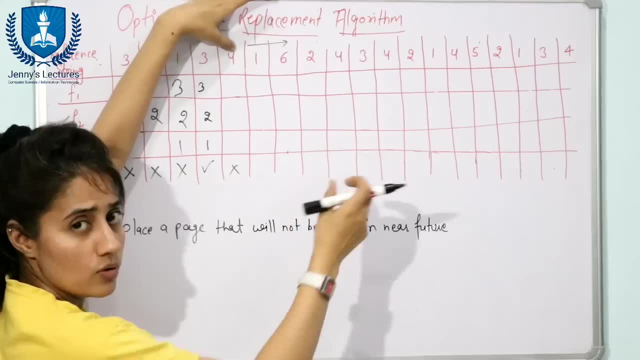 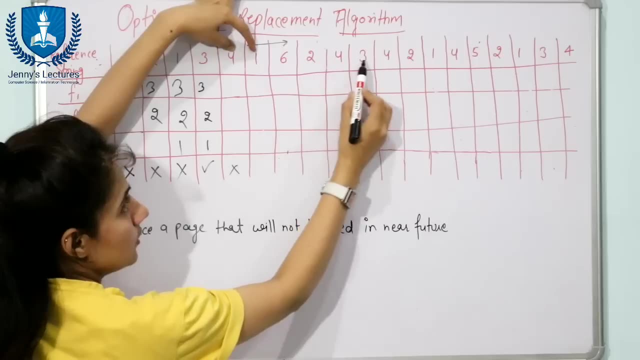 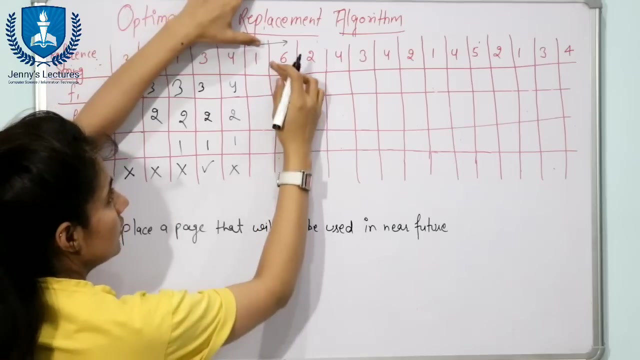 to the right, most right, most side will take that page. we will select that page as victim. so three, two, one. one is here, two is here, three is here, so we will select this. three here we will write four, then two and then one. now next is one, one is available. so this is a hit. four, two, one, six. 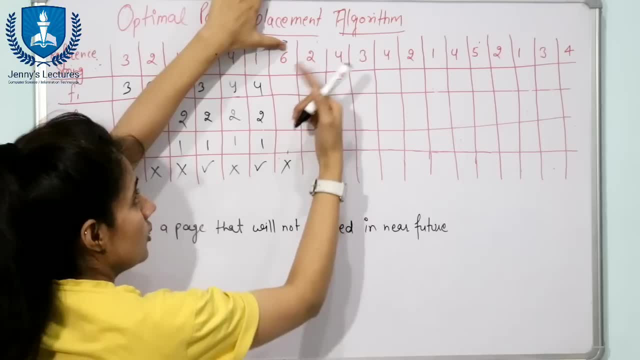 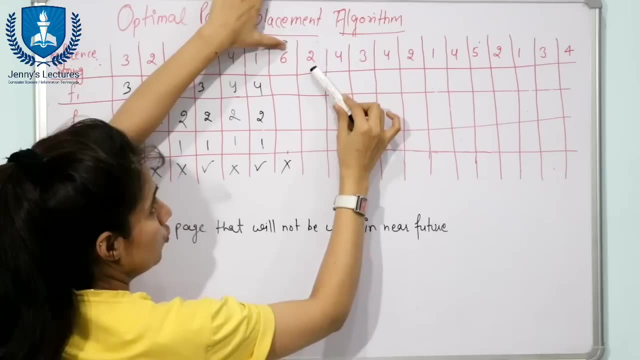 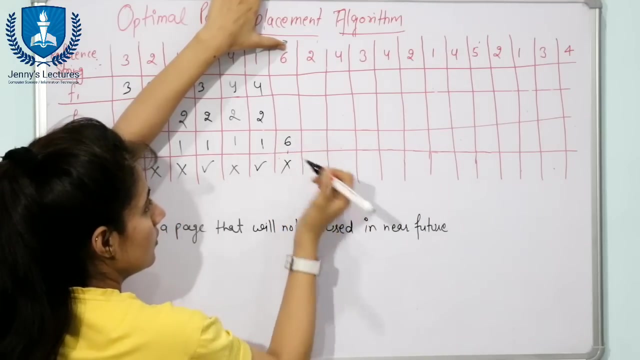 six is not available, so this is a miss. now check out, now trace out the string from left to right out of four: two, one. check out which pages to the right most part. two is here, four is here. one is here, so we will select one as victim. page one. here you will write six. one is to be replaced, two and. 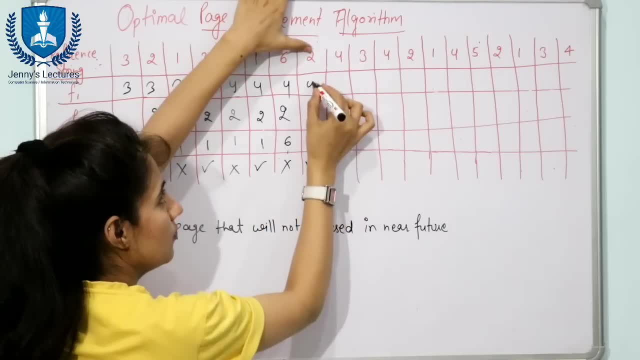 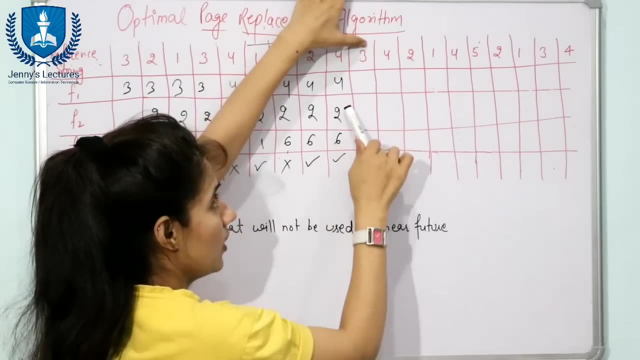 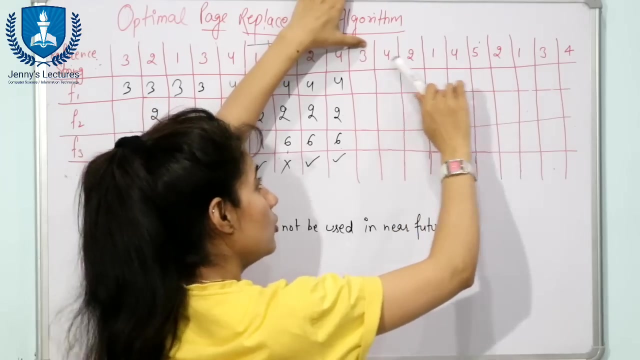 four, two, two is available, so this is a hit. four, two, six, four is available, so this is a hit. four, two, six, three, three, three is not available. okay, now check out in the future which pages to the right most part, which page is to be not to be used for the longest amount of time. here we have four. here we have two. 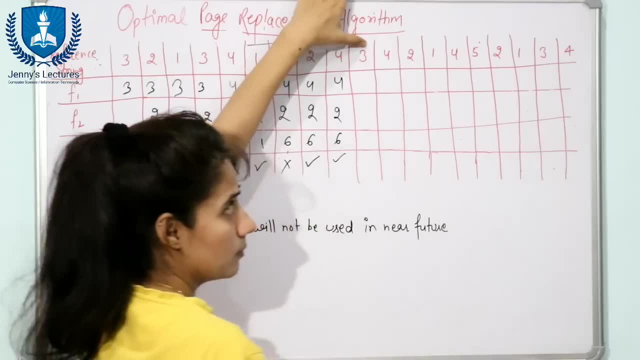 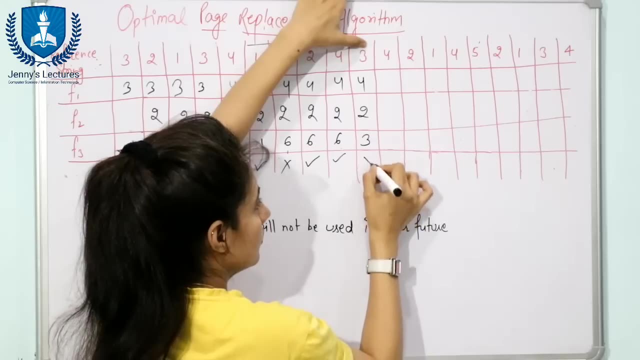 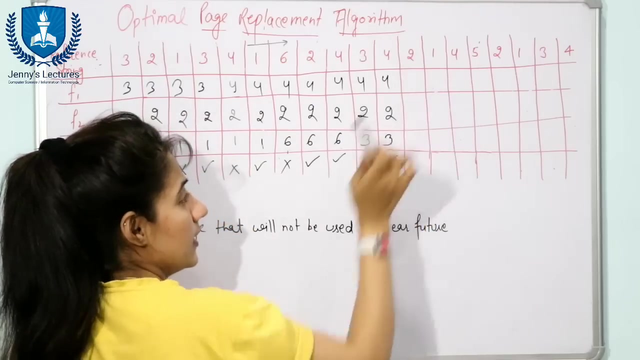 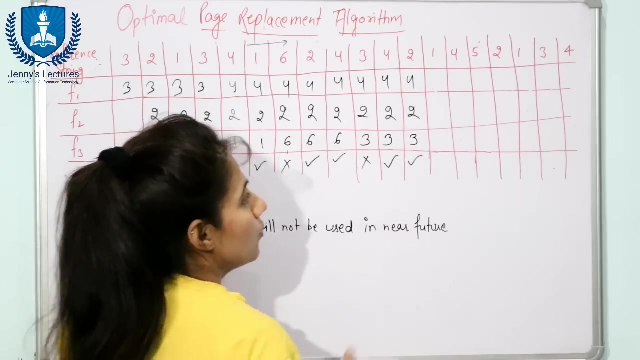 and six is not going to be used by the cpu, okay, so obviously we will replace this six. so here we will write three, two and four. here four, four is available, so this is a hit. four, two and three. next is 2. who is available? so this is a hit. 4, 2 & 3: 1, 1 is not available, so this is a miss now. 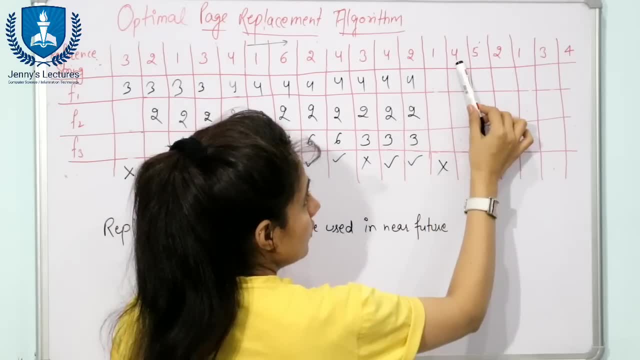 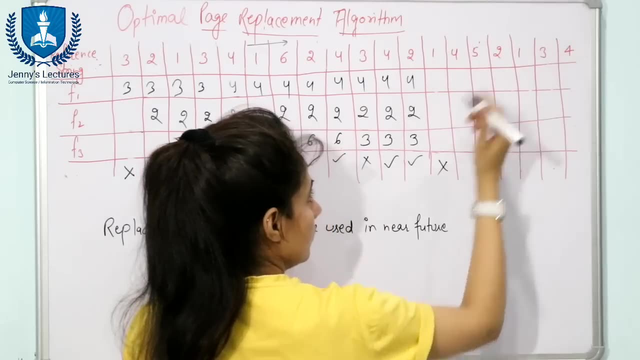 check out which is to be replaced out of 4. 2, 3. 4 is here. 2 is here. after that, 3 is here. so 3 is to the rightmost part, to the rightmost side. so we will replace this: 3, 1, 2 & 4. next is 4. 4 is. 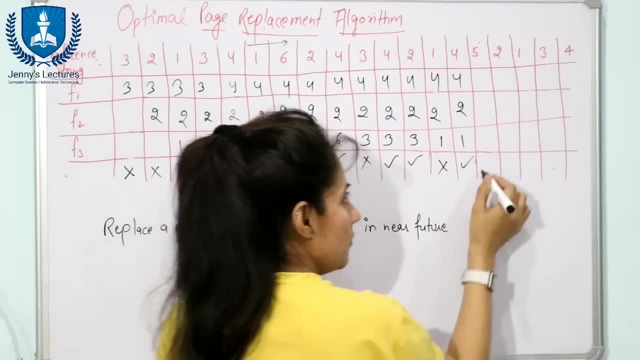 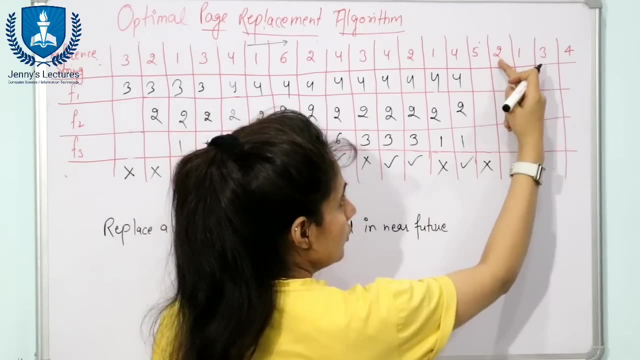 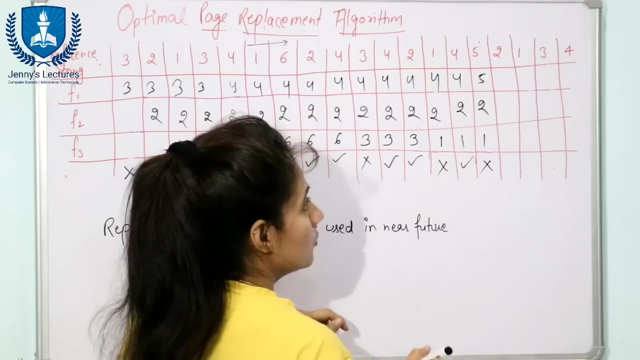 available, so this is a hit. 4, 2 & 1. next is 5. 5 is not available, so this is a miss. now, out of these three, check out which pages to be selected, as left them faced. four to one. two is here, then we have one, then we have four, so we will replace this: 4, 5, 2 & 1. 2, 2 is available, so this is a hit. 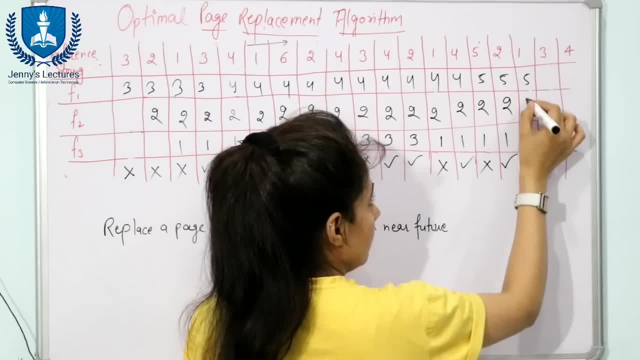 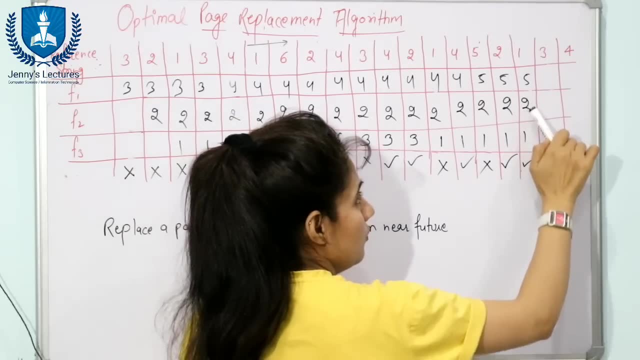 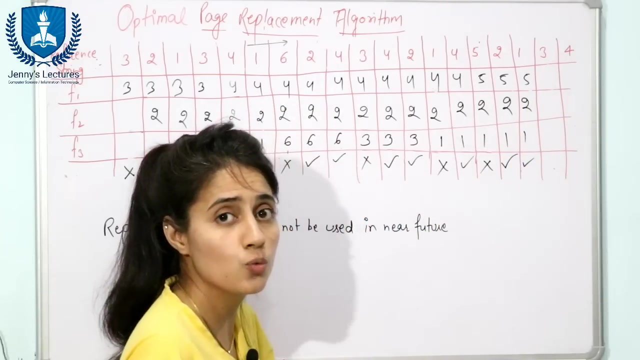 5, 2 & 1. 1 is available. this is a hit. 5, 2 & 1, 3. now 3 is not available. now which page is to be replaced? 5, 2, 2 & 3 to 1. see no pages out of these would be requested in future. now you will replace which page, so you. 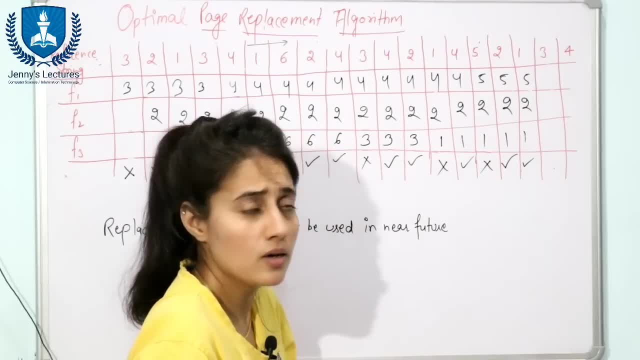 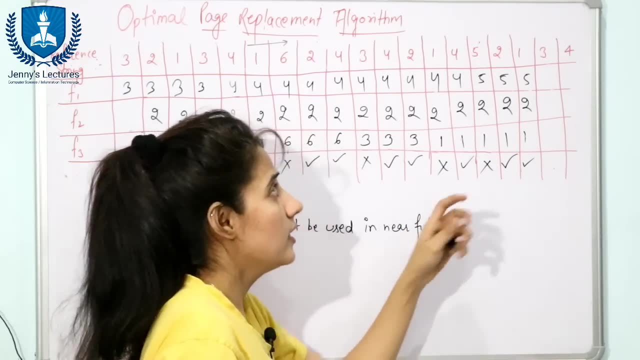 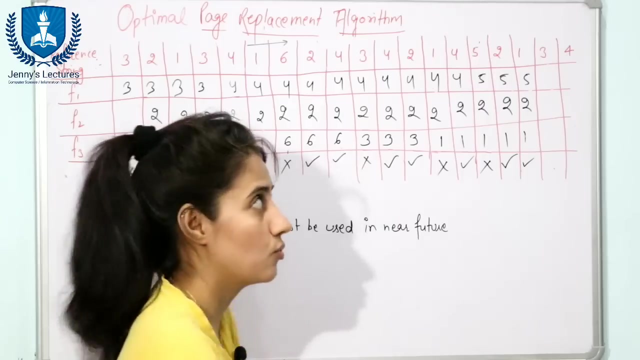 can select any one of these, because obviously it doesn't matter, because no page out of these would be requested in future, so we can replace any page. or you can say: in this case, if this thing happens, then we will apply what fifo technique first in, first out out of these three: 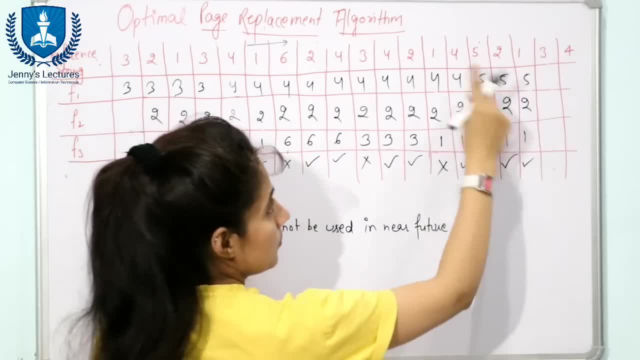 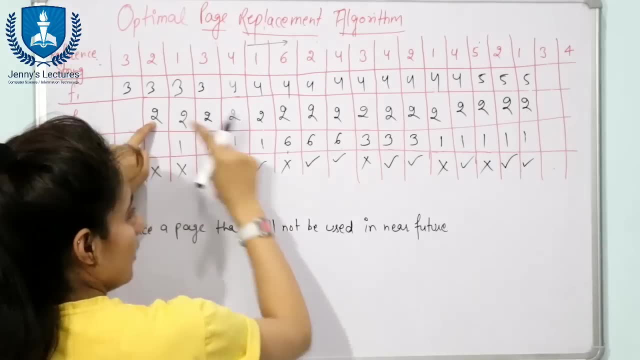 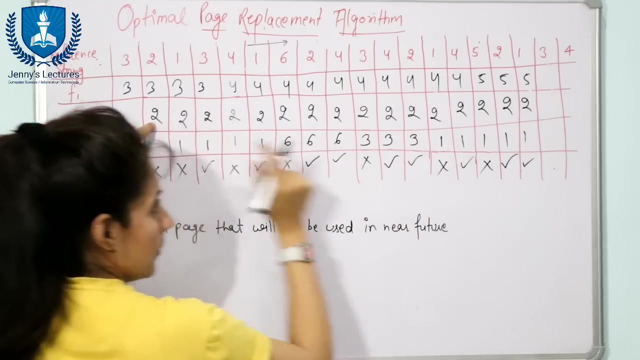 five to one, which is to be replaced. now, what was there in fifo? the simple trick is check out: initial point of five here, initial point of one is here, initial point of one is sorry. initial point of two was here and initial point of one is here, so this was the first page, so we will replace this. 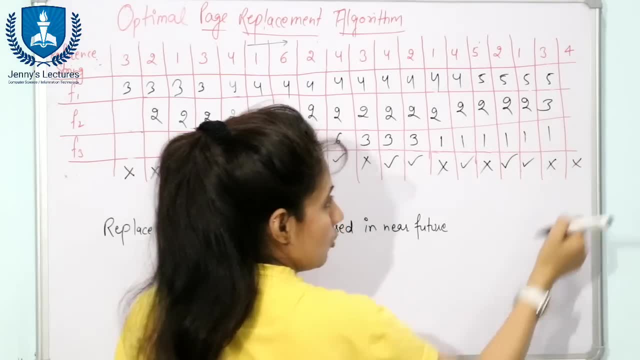 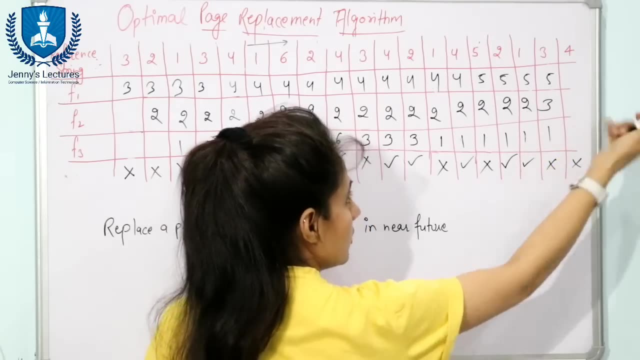 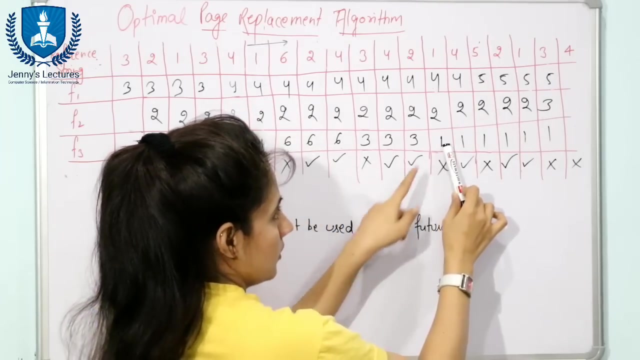 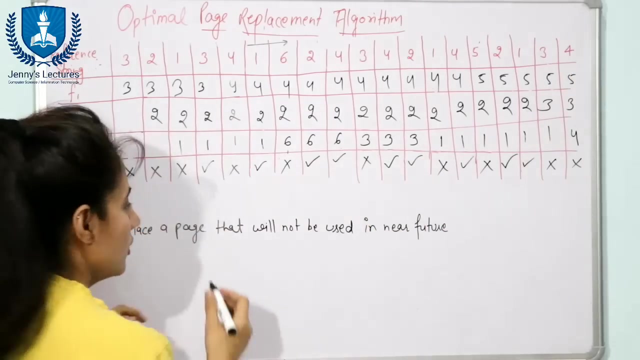 two, three, five and one. it is also a miss now: five, three, five, three and one. we don't have any future, any future request, so apply that fifo technique. five, initial point of five is here, three is here, one is here, so we will replace this one, because this was the first out of five, three and one. so here we write four, three and five. so 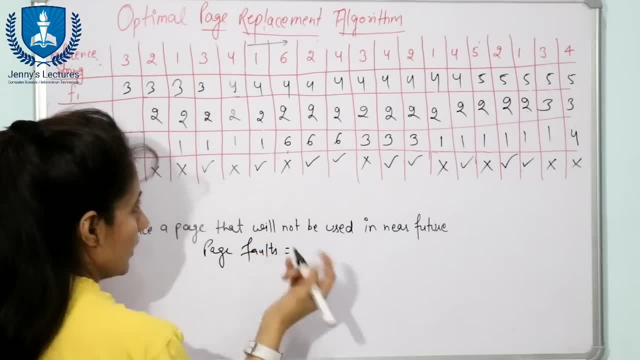 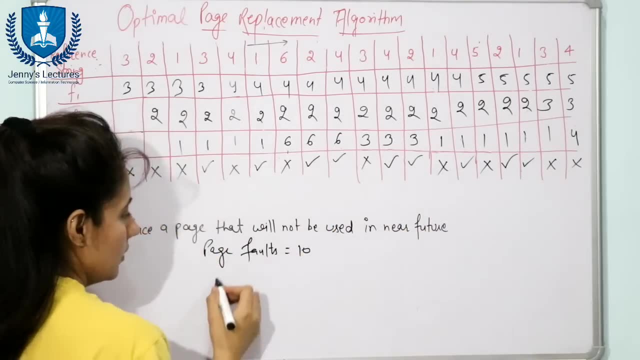 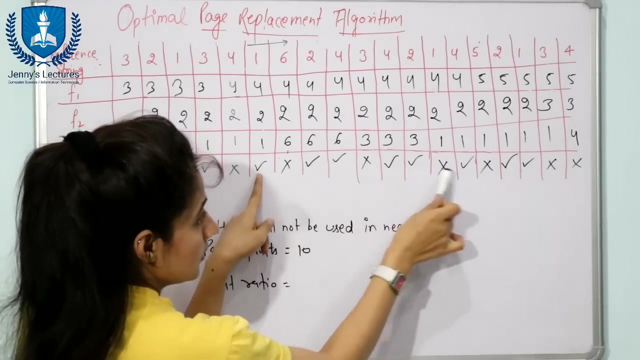 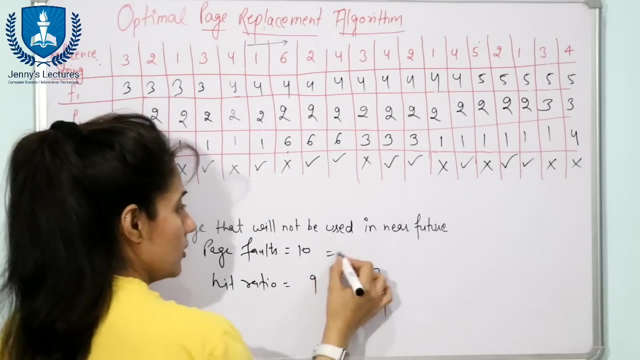 number of page folds in this case is one, two, three, four, five, six, seven, eight, nine, ten and hit ratio is number of hits. one, two, three, four, five, six, seven, eight, nine and hit ratio would be nine divided by total is nineteen, or miss ratio. you can say ten divided by nineteen, okay, so this optimal approach is. 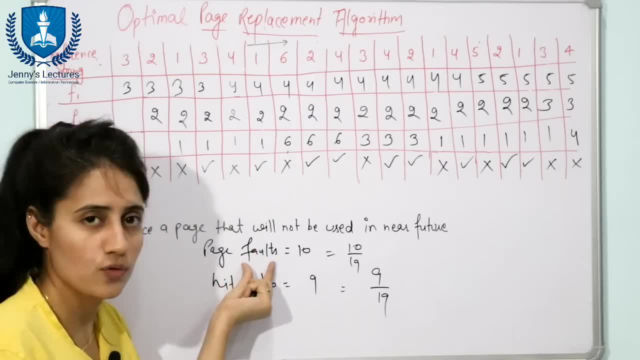 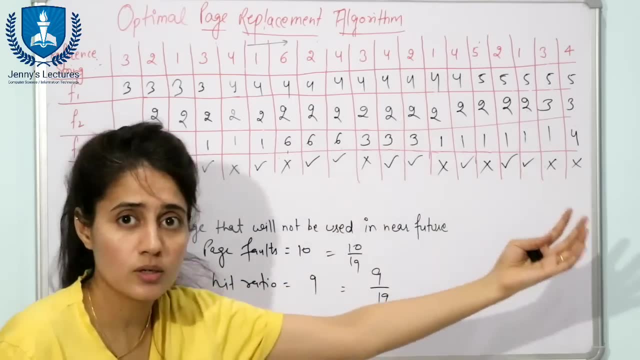 the best one. it will give you the least number of page folds out of all the techniques, although we cannot implement this technique. why so? because we are going to predict the future, and that is impossible. that is almost impossible. so it is very, very difficult, or you can. 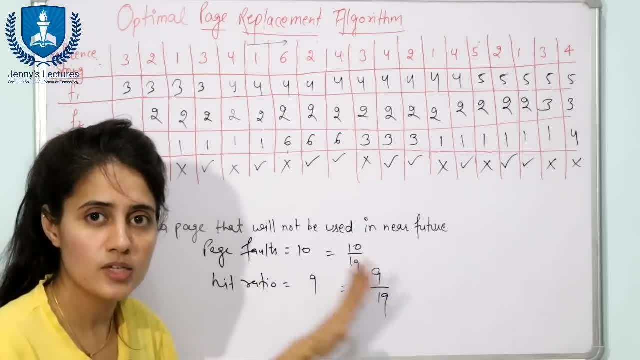 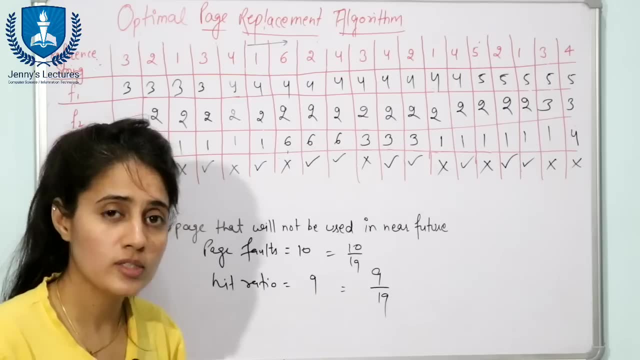 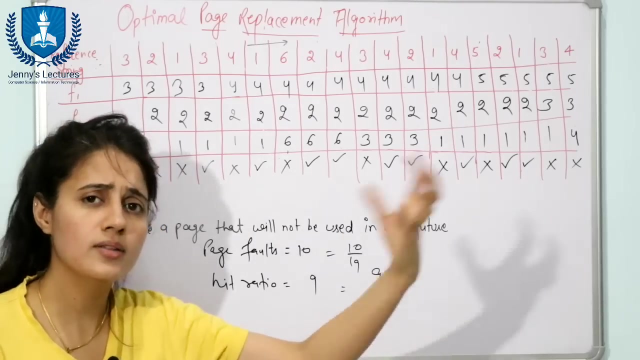 say almost impossible to implement this approach. now you will say: what is the use of this approach? because this, this is used as a benchmark. or you can say: this is to be used as a standard, to set a standard. we can, we can compare. we can compare all the other replacement algorithms. 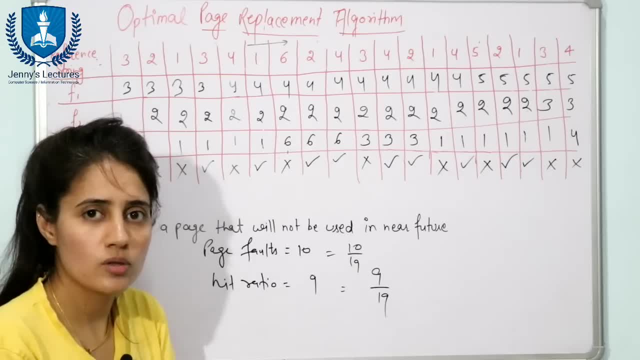 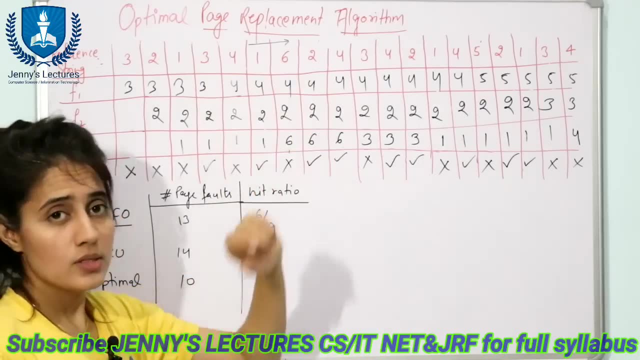 with this algorithm and you can say which algorithm is good, which algorithm is not good. so this is just for the comparison. this is just a theoretical concept. so now for this. give one reference string. if we compare the result of three techniques- that fifo, lru and optimal- then 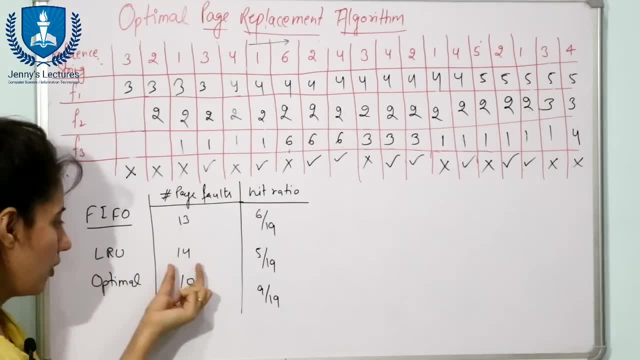 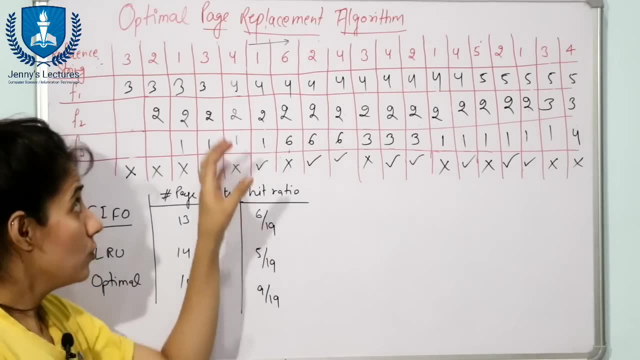 this is this. number of page faults in fifo was 13, in lru 14. optimal 10 hit ratio is 6 by 19, 5 by 99, 9 by 19.. so see, based on this, this data for this reference string, we cannot say that fifo is good. 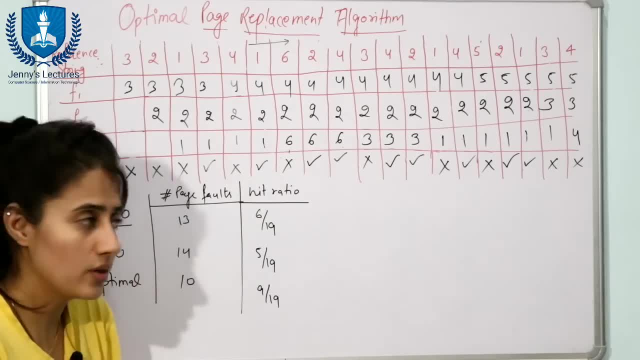 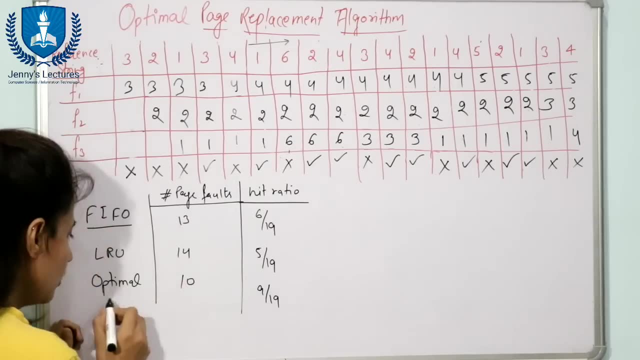 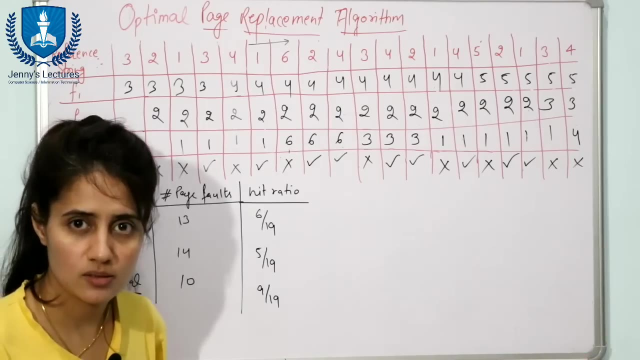 because it is given less number of page faults. maybe for some another reference string, fifo, will give you more number of page fault and lru will give you less number of page faults, but this optimal will surely give you the minimum number of page faults in any case. so this is you. 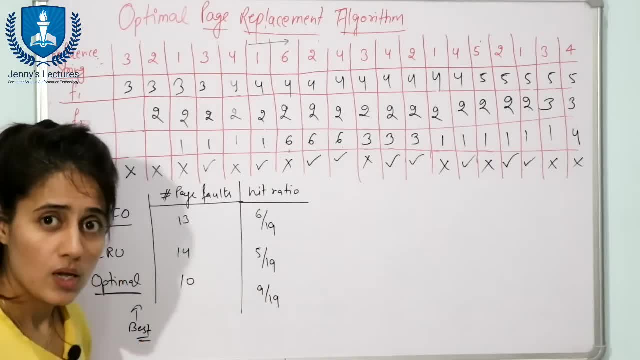 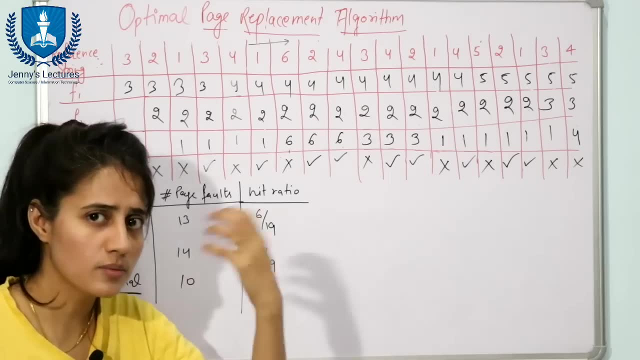 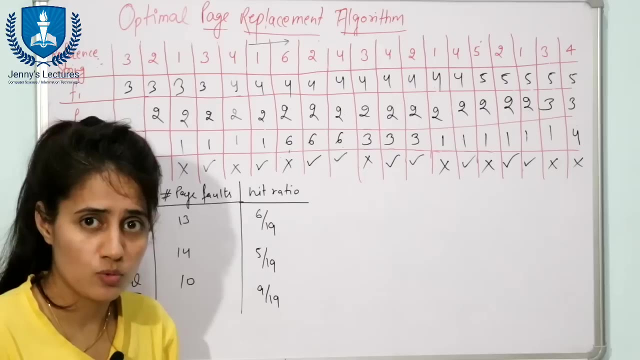 can say the best one. but problem is we cannot implement this technique. this is just a theoretical concept because we cannot predict the future operating system, cannot predict the future, that which the cpu is going to request, which page? that is almost impossible to predict. same drawback, as we have discussed in short: test job force.